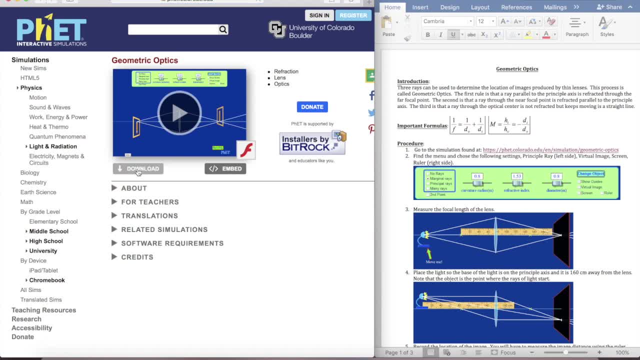 come up. Okay, so, as I say, it says I need to download it, So I'm going to download it. This is just a video, It's not the actual lab. Again, that's going to show up in my downloads folder, I can. 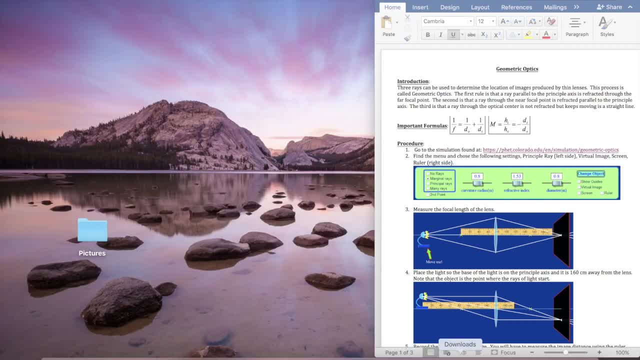 go ahead and close this because I won't need that anymore And I can see it right here. It's just kind of Here we go, So I'm going to click on that. It says it can't be open because it's from an. 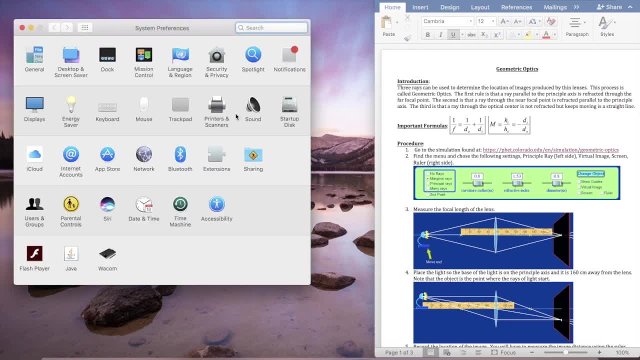 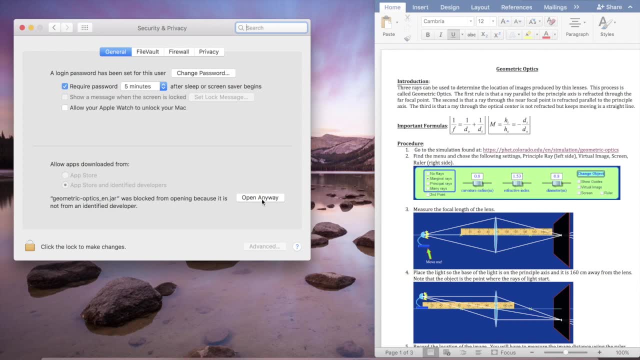 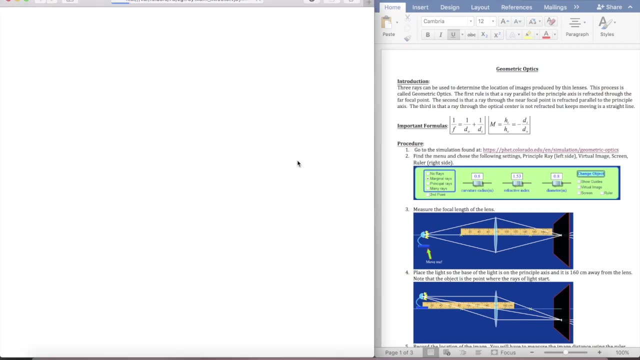 unidentified developer. So I'm going to go to settings and I'm going to go to security and privacy. It says, oh, it was blocked from opening because it's not from an identified developer. I'm going to say I want to open it Anyway. And it'll ask me: am I sure? Yes, I'm sure. And then here it is. Okay. this says they're. 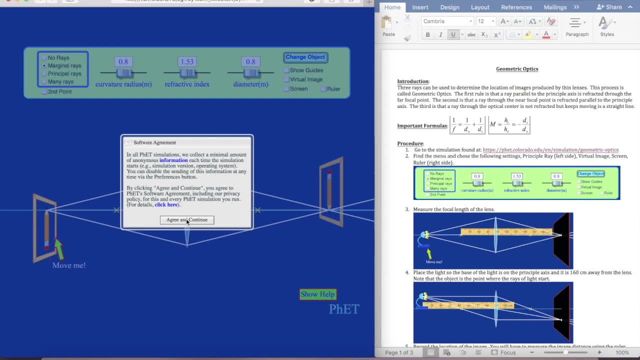 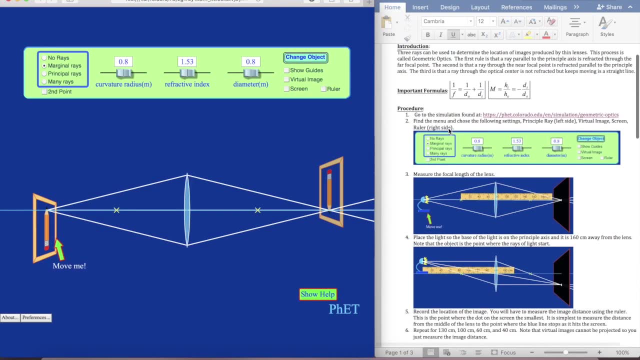 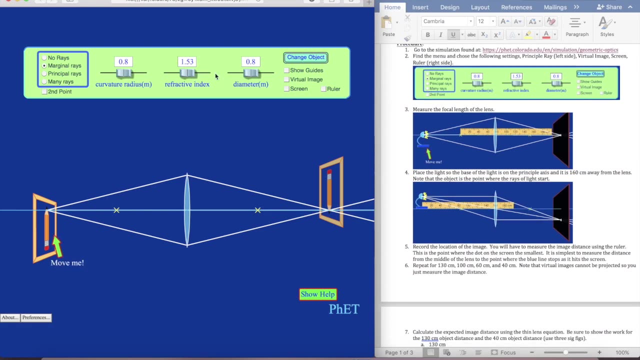 collecting anonymous information. You can disable this in the preferences, but agree and continue. Okay, so now I've got my lab and I can try and solve it. Okay, so it says: find the menu and choose the following settings: Principal Ray- It's right there- And then virtual image- It's on the right Screen- and ruler. 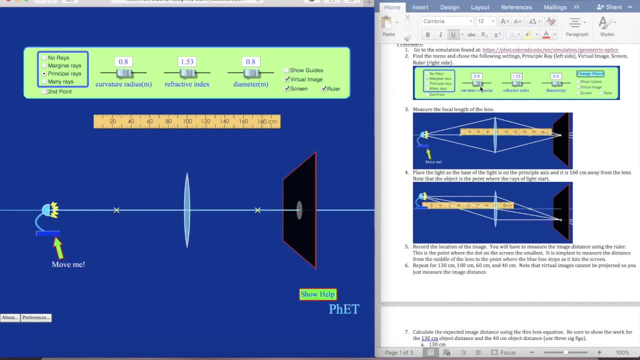 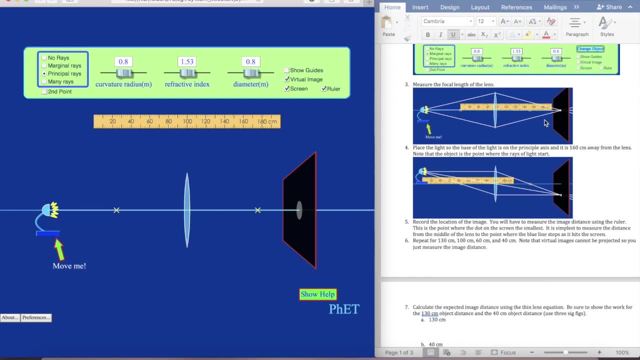 Okay. And then it says point eight, one, point five, three, point eight. Okay, So I'm good. And then it wants me to measure the focal length of the lens. Okay, so your focal length is three, this here. okay. so I'm just gonna kind of take my mouse point and I'm gonna move. 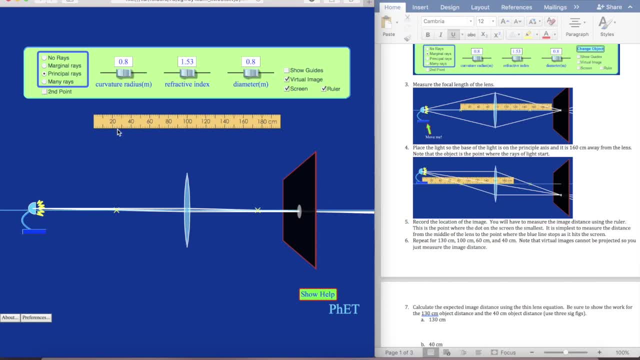 it up. I'm at like what? like 24, so it's 24 and 100, so basically is like 100 minus 24, okay, so I'm just gonna write this right here so I don't forget it, so it can be 76 and that's in centimeters. okay, now we want to place. 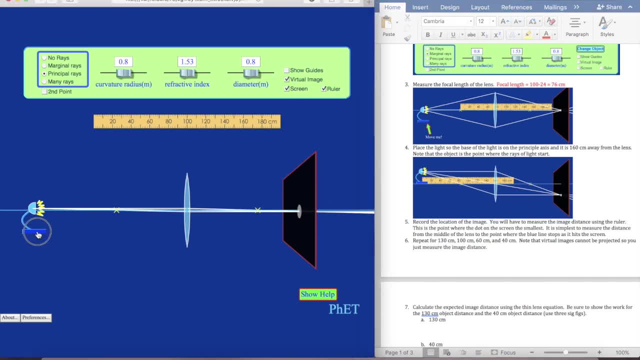 the light where the base of the light is on the principal axis, so I want this light to be right here, okay, um, oh, we can also move the ruler down. oh, that's nice, that would have made that a lot easier. huh, so it looks like I was right, though. um, sorry, I'm gonna keep it. 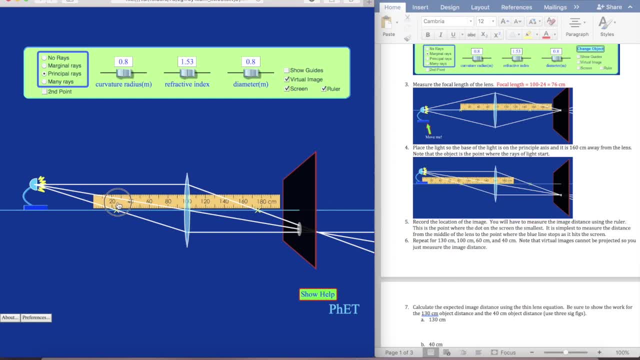 in the middle. I think that's just gonna make it easier. there we go. okay, and we wanted a hundred and sixty centimeters away from the lens. okay, so 160. it's right here, and I want the light, the actual light, 160 centimeters away. oh, look at that, that's basically where I was. that's handy, okay, right so. 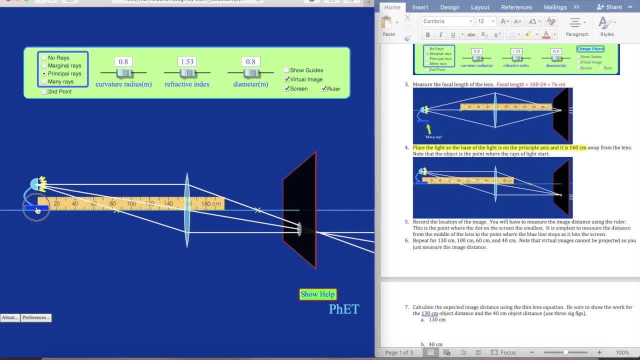 it's where the the rays of light start. so they actually have the rays of light a little bit down, okay, and so we want to bring the. finally, because this we're going to vacuum- like, how many of the lines do I have on there? and we just gotta got this. 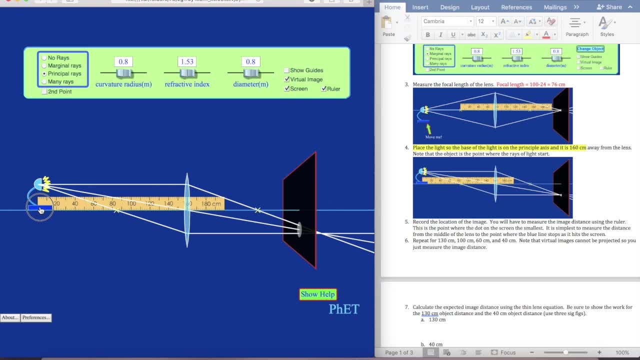 out of here, go a little way around, okay, so let's. okay, so we have. I'm gonna slice this little bit down, let's see if that fits right in now. allowing the color to blend left side of the pipe. also in just a little bit for the shape, but it doesn't bother you. 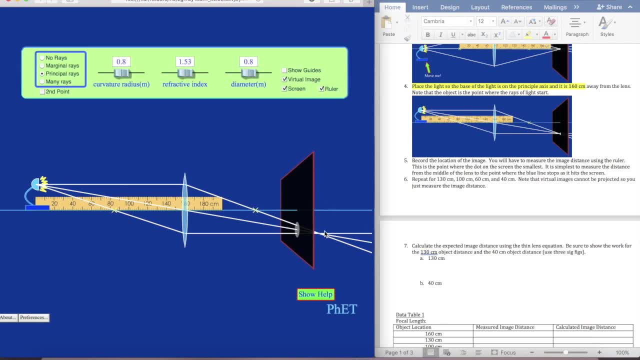 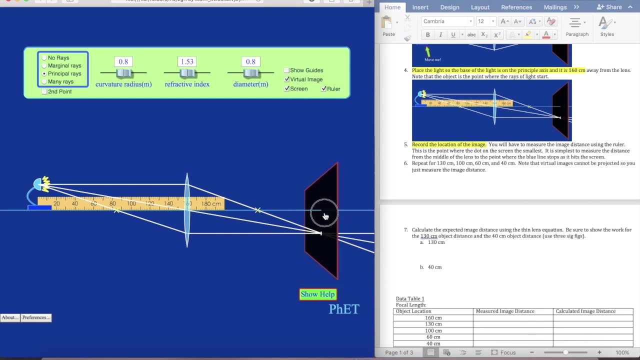 okay, now we want to record the location of the image. okay, so the the image is going to be where these intersect, right here. okay, so this is what they said. they said it's where the dot on the screen is the smallest, which also happens to be right where they intersect. okay, and then I'm gonna need to measure this, okay, so. 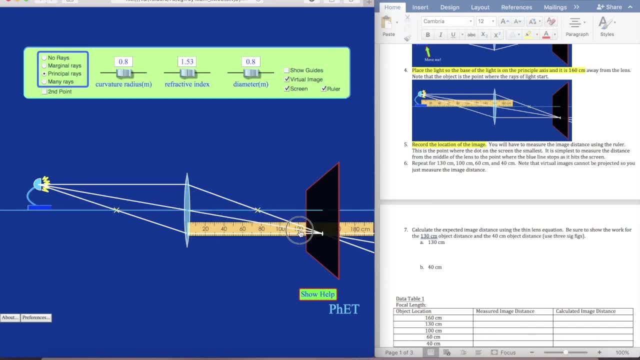 I'm gonna go. I have to start from the center of my lens. well, that's annoying that the ruler goes behind the screen. that's frustrating. I'm gonna move this screen all the way, because it's just where these intersect, right here. okay, so what is that? 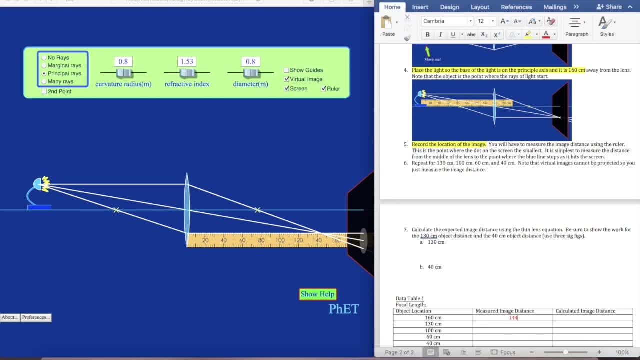 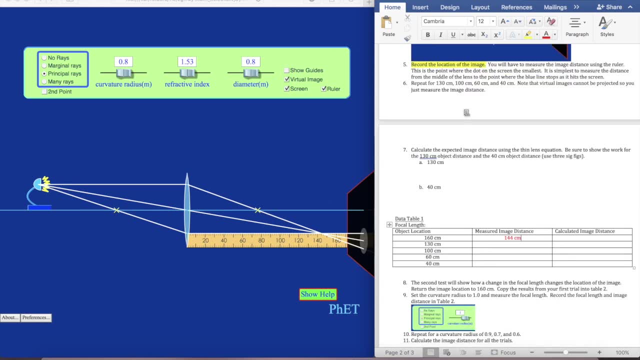 so that's where these intersect, back here. so it's at this point right here, and I'm gonna measure that. so I've got that on the screen, okay, and the distance between these two filters is going to be about 144, okay, and I'm putting that in my data table, okay, and then we're gonna repeat it for 130. 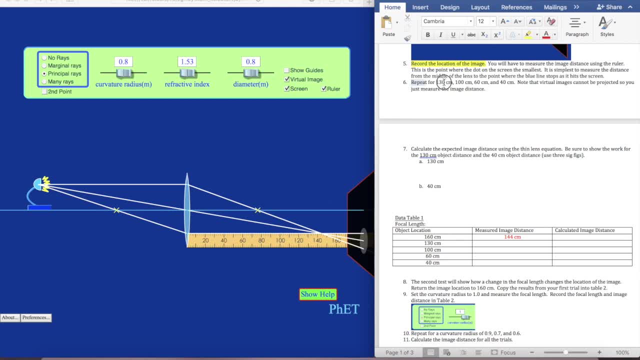 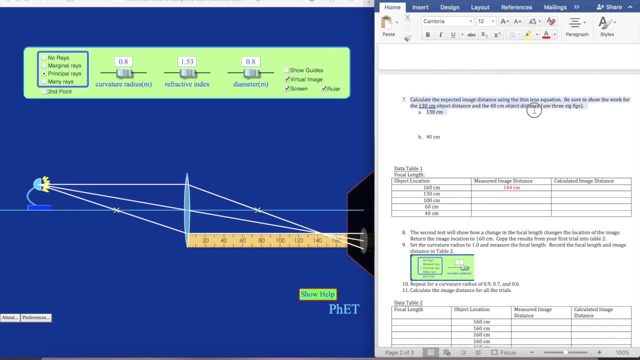 centimeters, 100 centimeters, 60 centimeters and 40 centimeters. virtual images won't be projected, so you'll just measure the image distance. okay, so that will. when we get there, I'll show you what that looks like, okay, and then we're gonna calculate the expected image distance using the lens equation. and then we're going to calculate the expected image distance using the lens equation and show your. 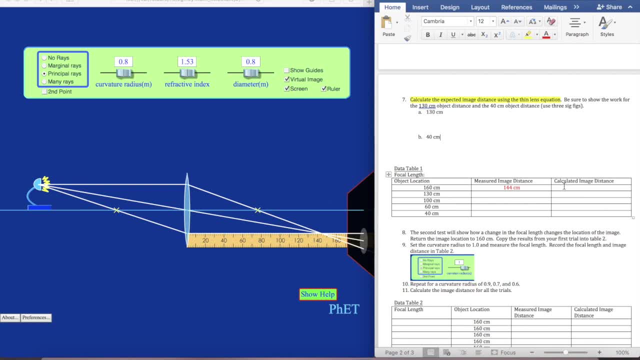 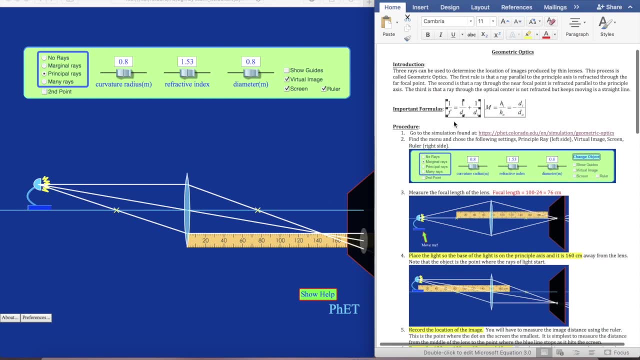 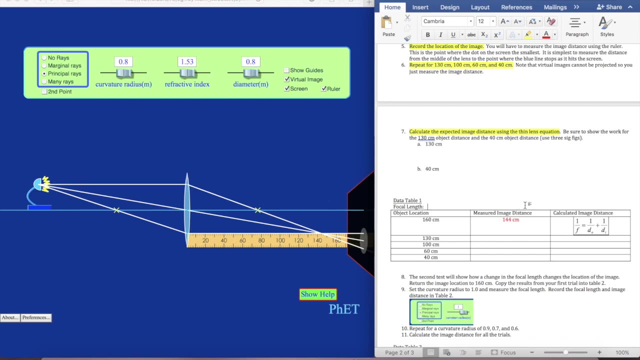 Show your work for 130 centimeters and 40 centimeters, okay. So to calculate the image distance, you're going to need to use this guy. Okay, and then you have your focal length. What did we do? We wrote it up here: 76 centimeters. 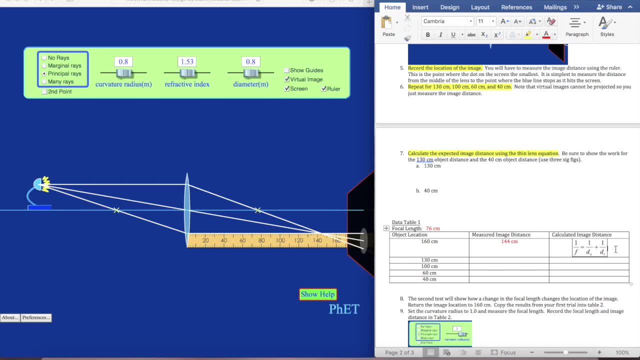 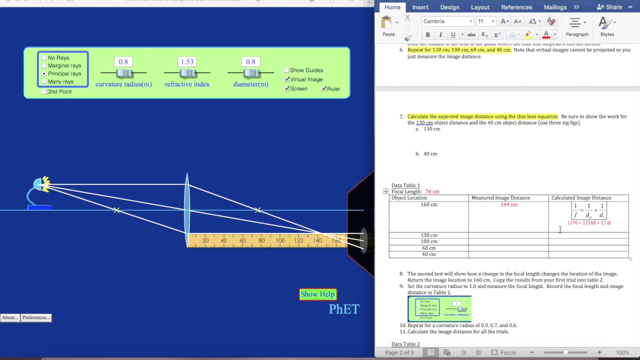 So we'll have something like 1 over 76 equals 1 over 160, plus 1 over di. Okay, I'm going to do 1 over di equals 1 over 76.. Okay, and now keep in mind, this is really important. 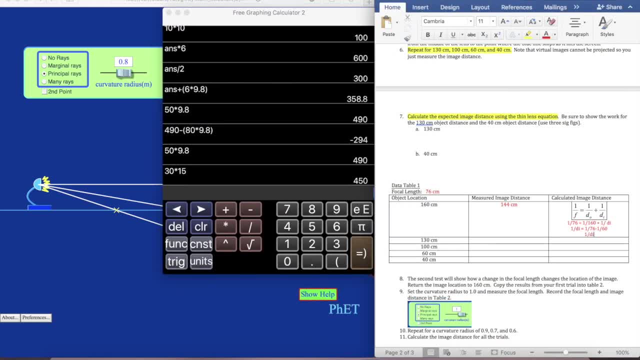 A lot of students make a mistake here. Okay, so we've got 1 over di equals 1 over 76. So I'm going to do 1 divided by 76 minus 1 divided by 60. Okay, And I'm going to get a really small number. 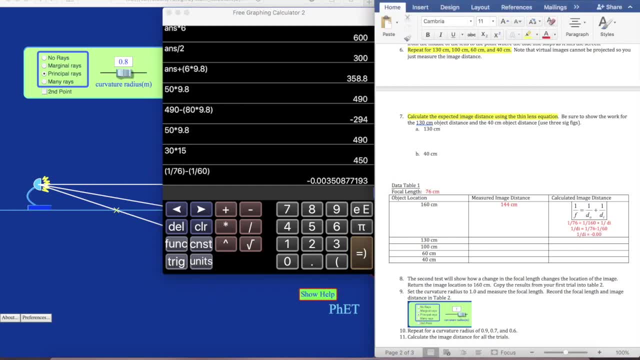 Okay, Okay now, in order to get the correct answer. okay, I need to move, because this is 1 over di right, So I need to do di equals. so I'm going to move it to both sides. We're going to do 1 divided by negative .0035.. 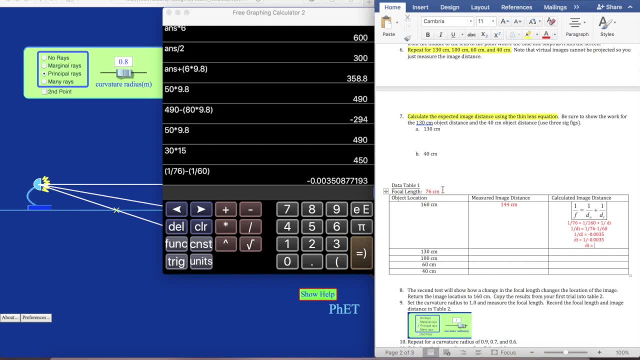 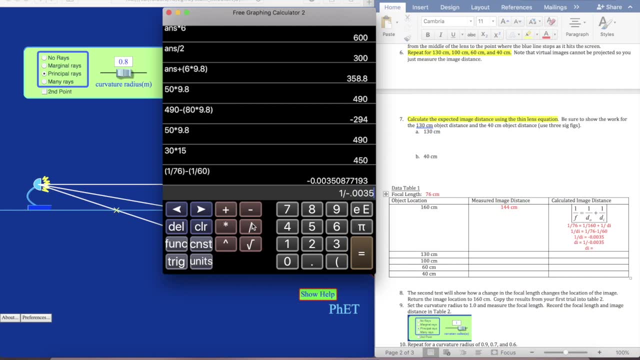 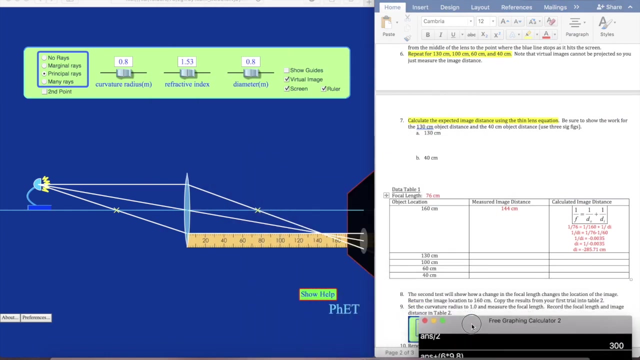 And you have to do this in order to get di, Otherwise you're not getting the right answer. Right, You're just getting negative 285.71.. Okay, now, that is interesting. That seems a little different than what I got. 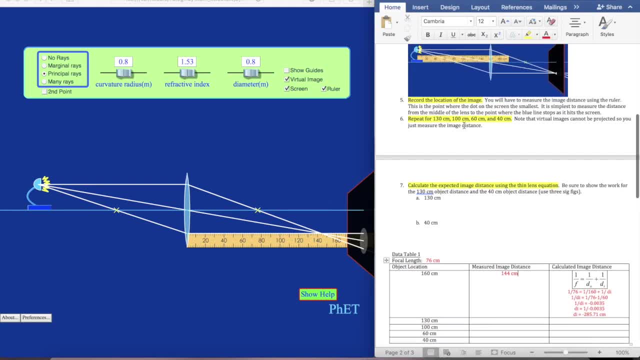 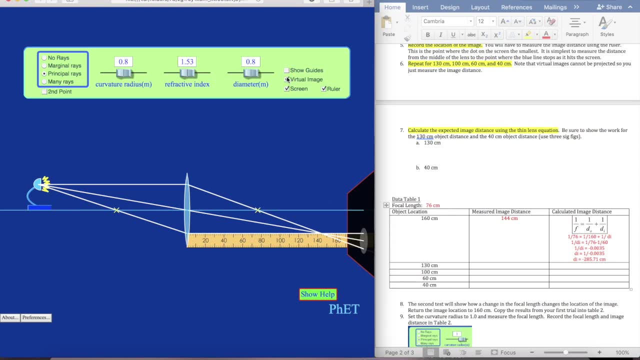 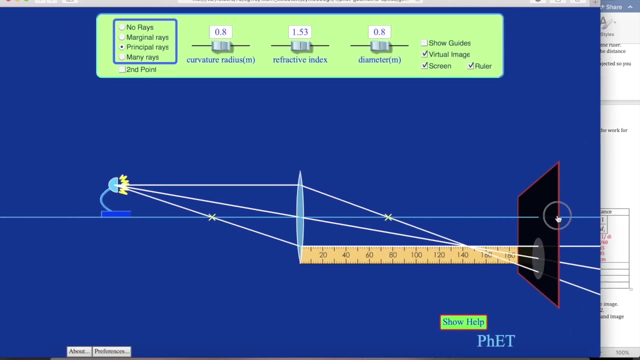 So I'm going to look at this and make sure that I'm okay. Okay, virtual image. Let's see I'm going to pull this bigger, just to make sure. Okay, we need this very small dot, remember, Remember, Okay, so I have 120. 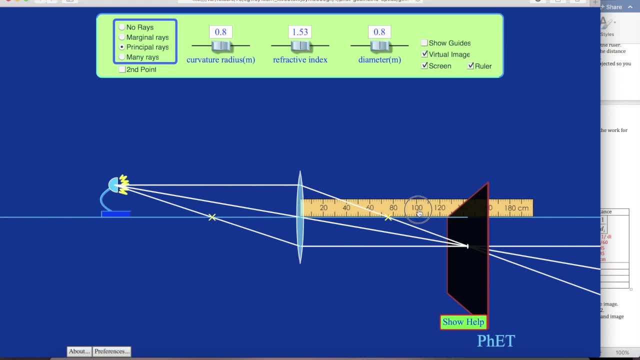 So they suggest measuring this blue line where it disappears, which is still kind of hard to see, Right? so I think this is actually easier. So it looks like what? 144.. Okay, And then let's see, let's make sure this is 160, yep, okay. well, that's what we've. 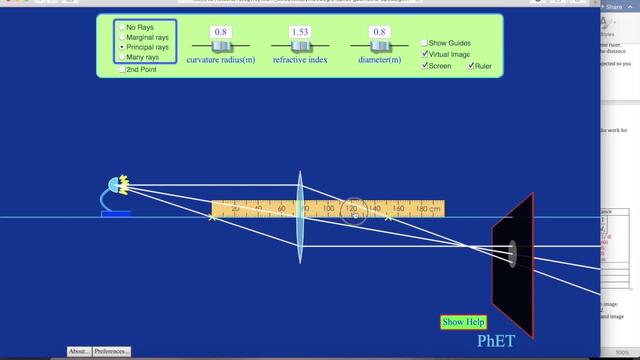 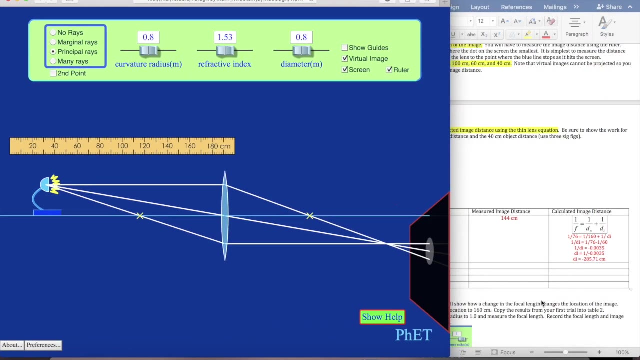 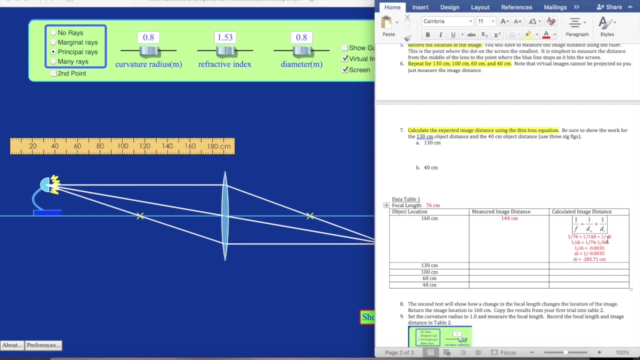 got. And let's see our focal length. make sure we got that correctly. that's 7246, 76, okay, so we um, Okay, We got it correct. um, oh, I see what I did. look what I did here um check this out. 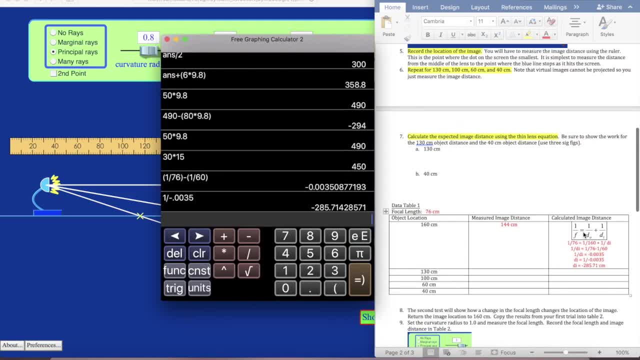 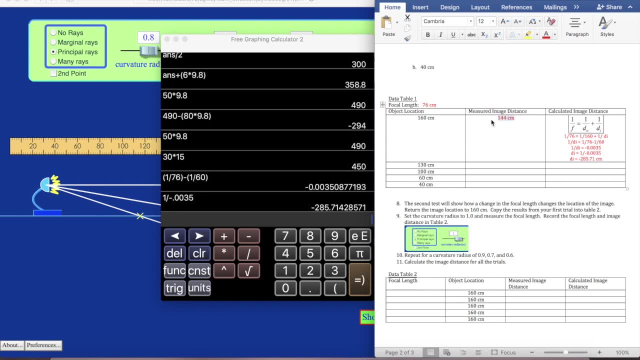 this is important, okay, because you guys might make a mistake like this too: um, you know, when you get an answer and you go, hmm, that doesn't seem really right. right, because it's not the same um, or not even close. 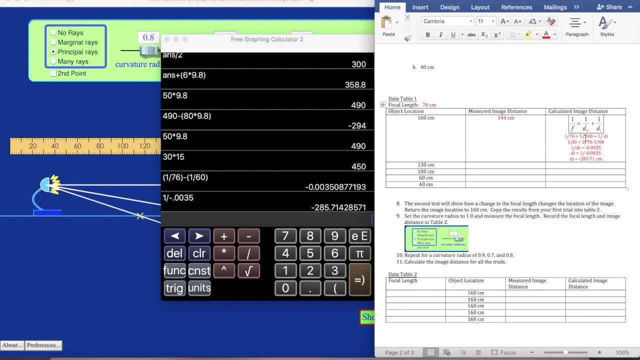 So let's look and see, see how I have: 1 over 76 equals 1 over 160,. well then, here I just put 60, so it needs to be 1 over 160, right? So that's why my answer is wrong. 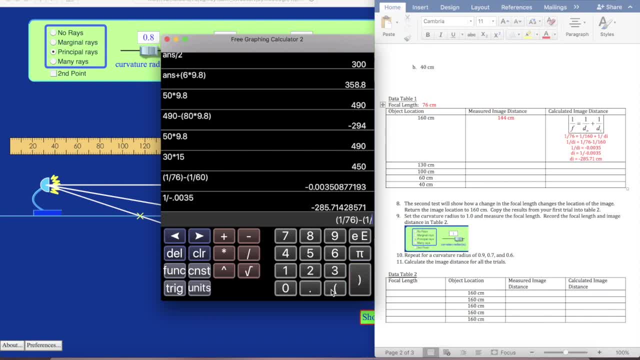 So let's try that. Okay, so this is going to give us a completely different number, Okay, And it's a positive number. do you see that? Which makes more sense to me, because a negative number would mean that it would be on this: 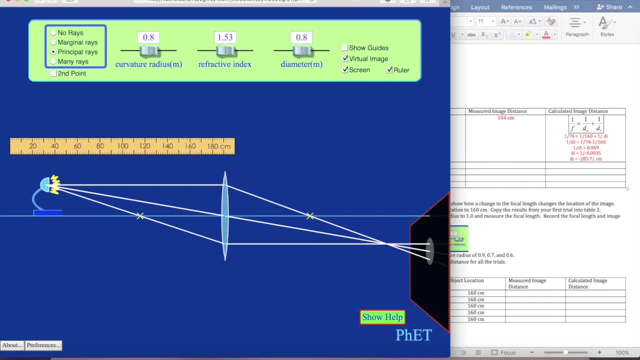 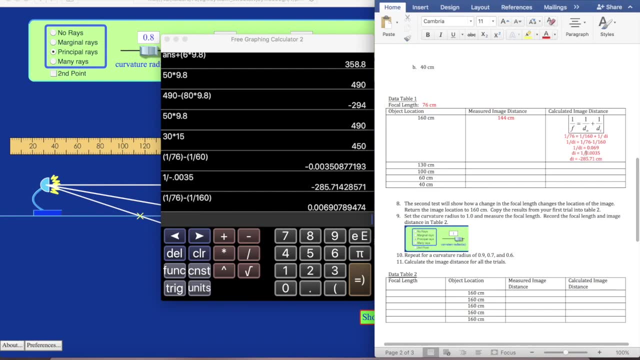 left side, the same side as the light, and see, it should be on the right side. so that should have tipped me off, but I was going with it, Okay. so I'm going to change this to this .69 again, and then let's do 1 divided by: 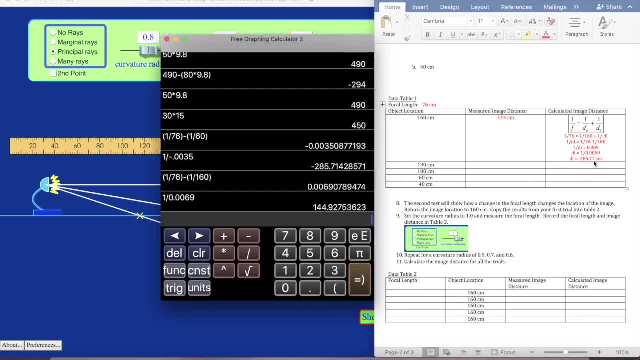 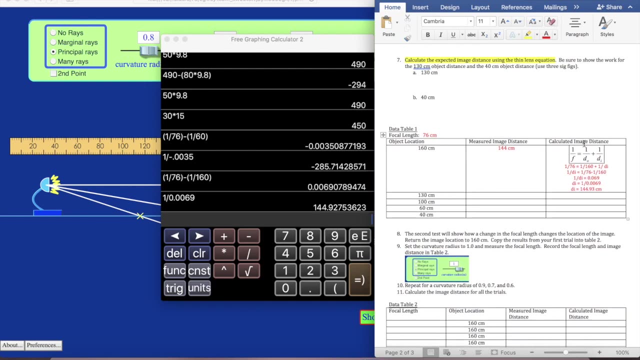 0.0069,. see what that is. Look at that. Look at that 144.93.. That is so much closer right. That makes much more sense. I feel much better about that, okay. So that's kind of how you'll solve these problems, okay. 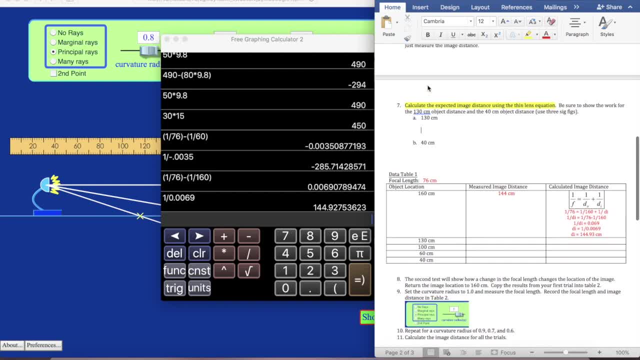 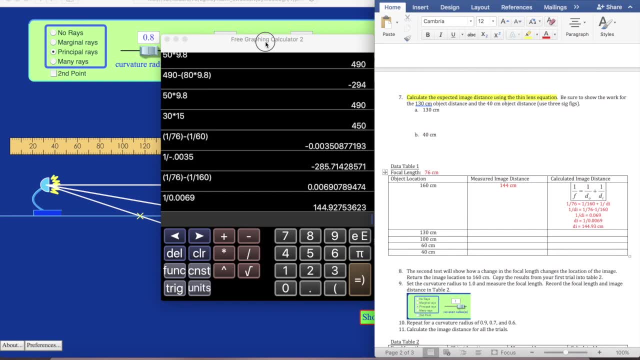 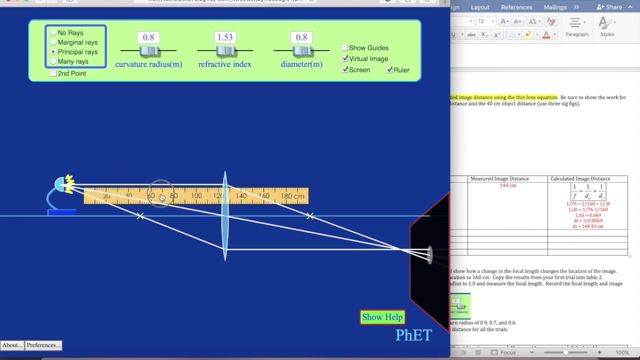 And you need to show your work for the 130 and the 40,. okay Now, um, let's try another one, Let's do, let's do, uh, 60, just to see what happens. Okay, So this is a virtual image. um, so I want to see which one will work. 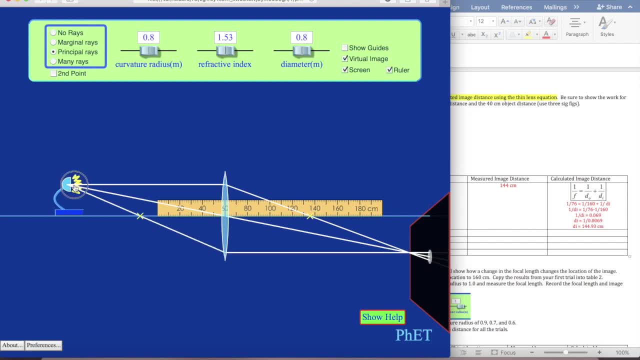 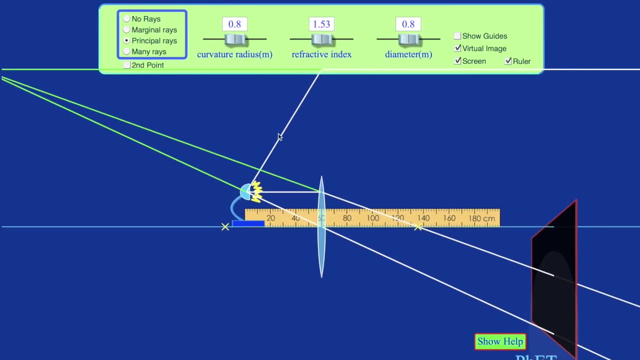 So we want 60 centimeters away, so I'm going to move my light until it's right here. Okay, do you see what happened here Now? um, let me see if I can make this larger. Okay, So at 60, we've got, um, we've got 60. 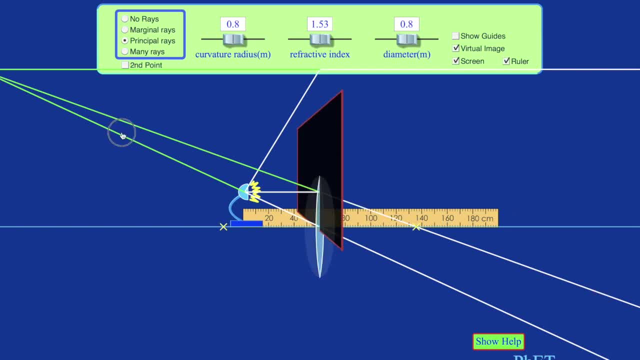 Okay, We've got the light rays coming back here and they are going to meet somewhere back here, which let me see if I can change the preferences. um, okay, um, so that's not going to work, So we're just going to have to kind of guesstimate a little bit. um, so this is. this is 200, right? 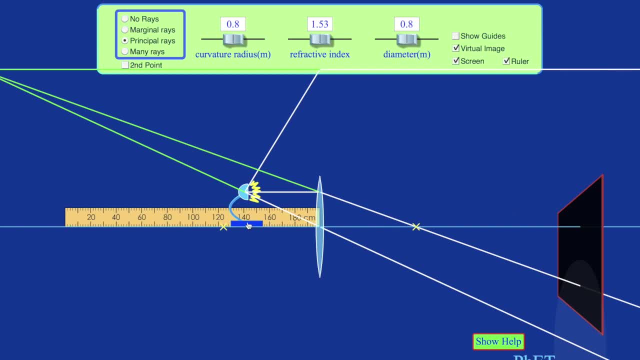 here, okay, And then, um, I'm trying to think of a way that I can. I'm just going to put my hand on the screen right where this is, so I know where to move it to, Okay, and I'm just going to kind of guess where these might meet, maybe like that. 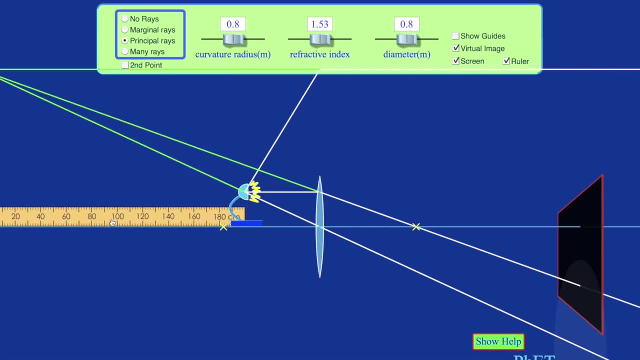 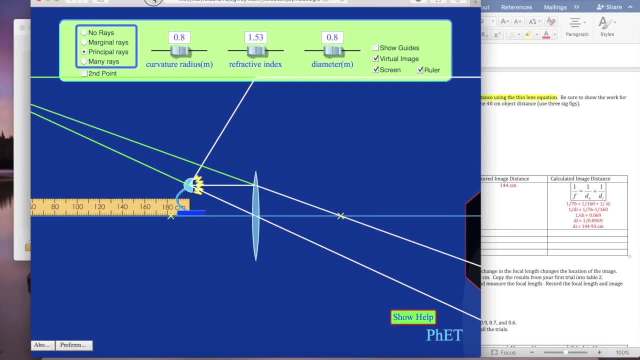 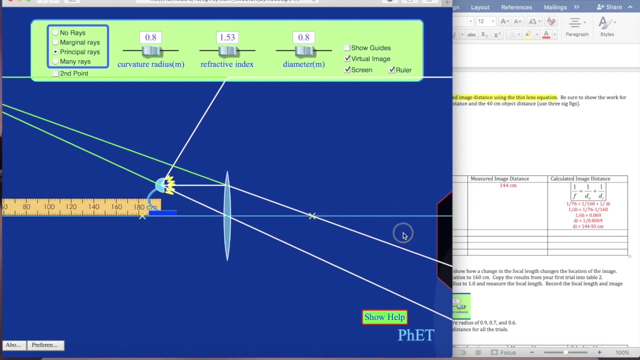 Okay, so I'm going to do like 260.. I don't know if that's right, Um, you know it's hard to tell Because it goes all the way to the edge there and they don't let you adjust this, um, but 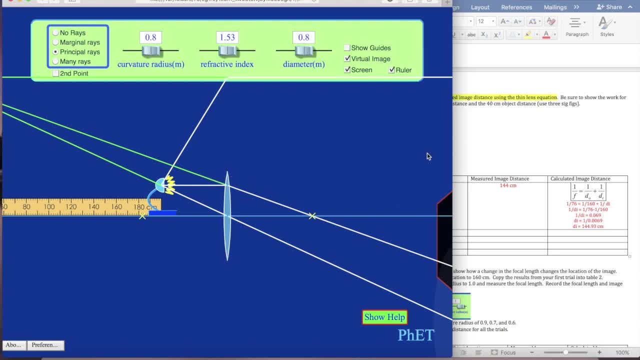 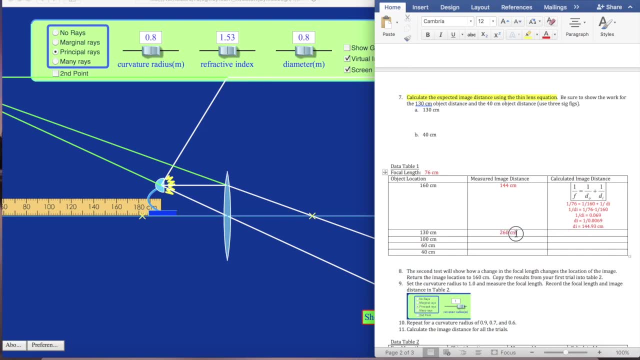 we'll try um 260, I think that's confusing, that doesn't help. Okay, So I'll do 260 as my image distance, and then, oh, that's not for that one, And then I'm going to do um. I'm going to do the math again. 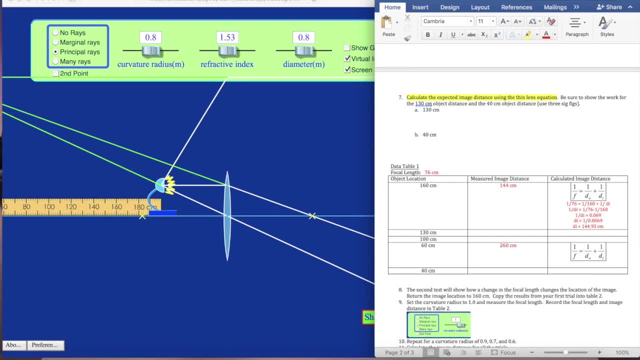 Just so we can see if we got it kind of right. So um this should be: 1 over 76 equals um 1 over 60 plus 1 over di. So we have 1 over di equals 1 over 76 minus 1 over 60, and we have 1 over di equals do. 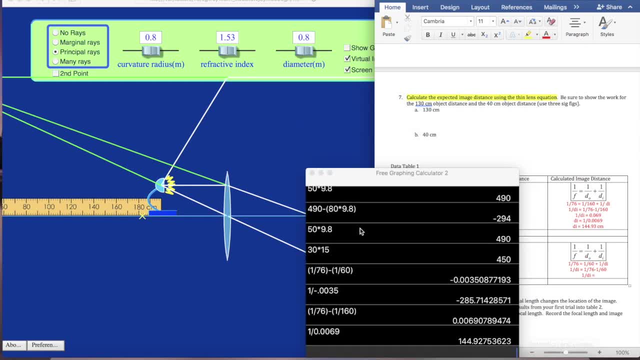 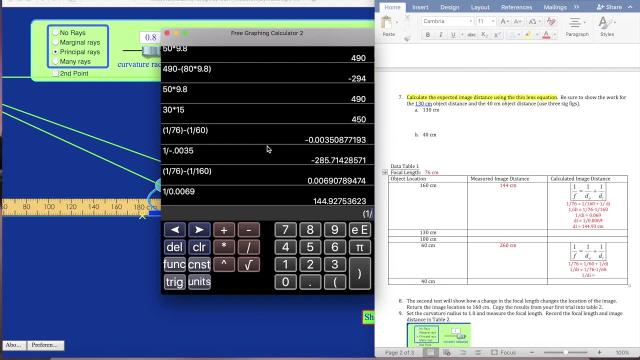 you see, I copied what they had here and I just put my new numbers in. Okay, Now look at this. This is actually. this is kind of funny. This is what I put before, right, when I did it wrong for the first one. 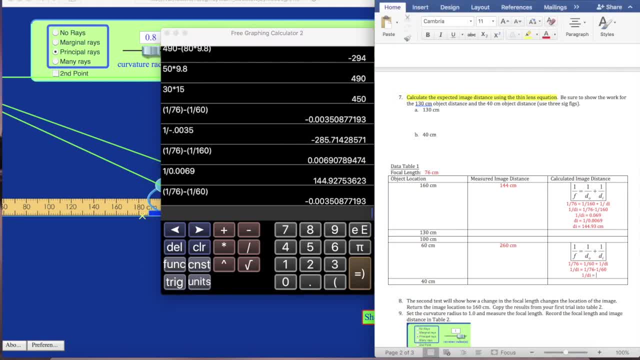 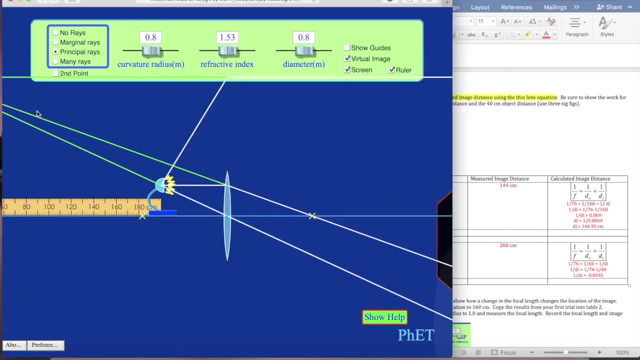 So we'll get a negative, And that's actually okay, because that's what we want, Because you see how our image, where it looks like the rays are coming together, is on the same side as the light. That's what we want. 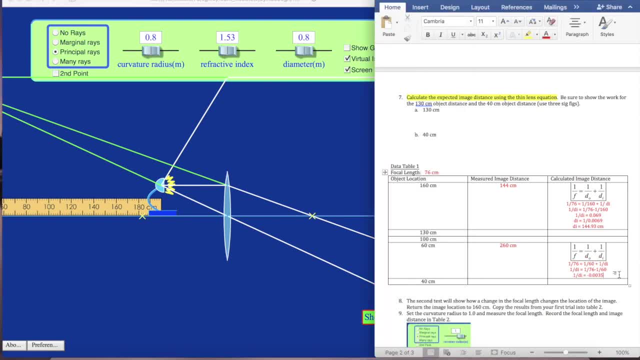 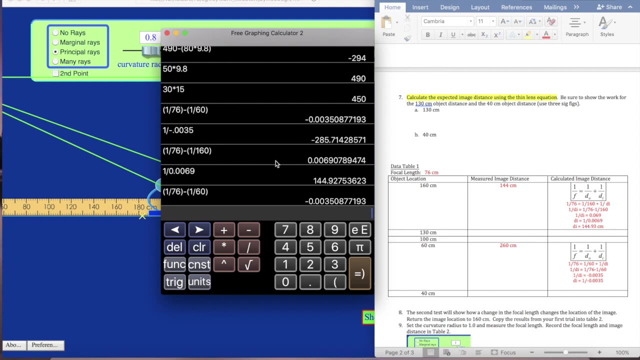 Okay, That's why we're getting that. That's what that negative means, okay, And so we're actually getting what we're supposed to get for that. So let's see Where's my calculator. I'm going to have it run over. 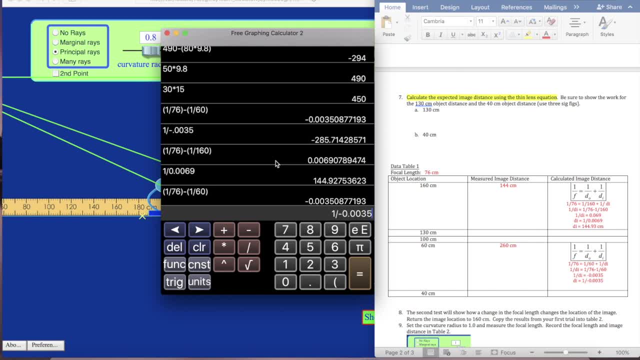 I know I did it before so I could just look up, but I'll do it again. Okay, negative 285.. Now it's not as close as the last one, but remember the last one we were actually able to measure. 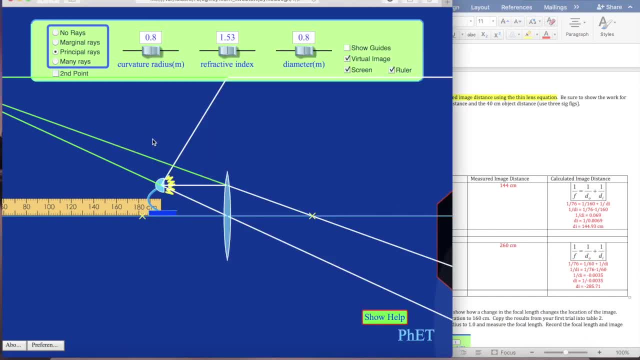 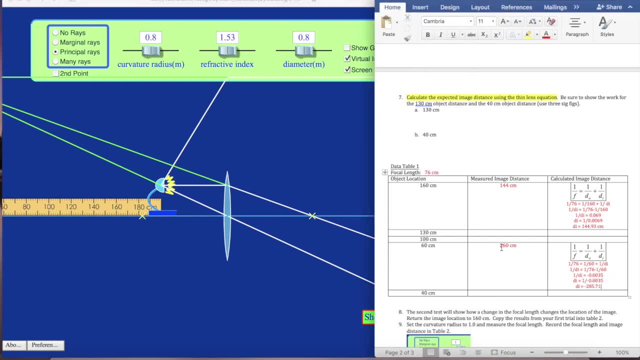 where this one. we kind of had to guesstimate. So 260, 285, that's not too far off, I'm okay with that and that makes sense, right. It's at least, like you know, above 250,, below 300,. 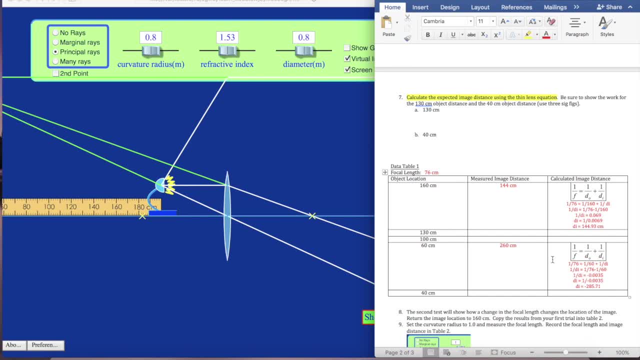 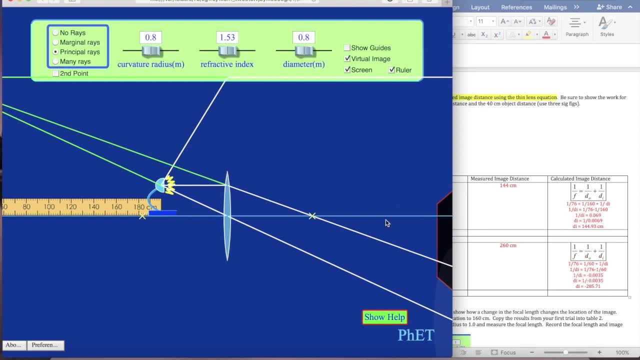 and the sign is correct for the right side. So that's kind of how you'll do those. And, like they said earlier, that's a virtual image and so that's why this little screen here. you know, nothing's showing up on that screen. 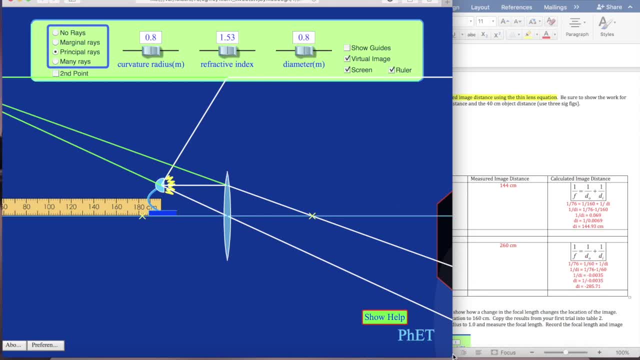 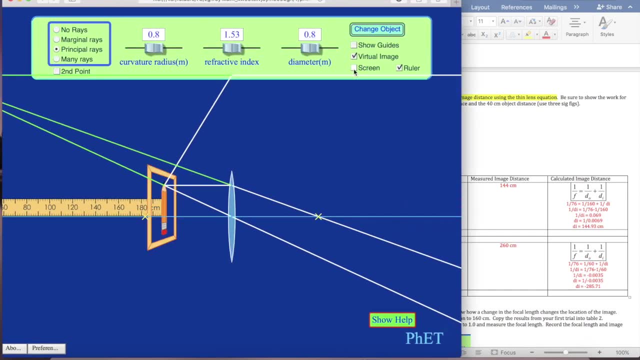 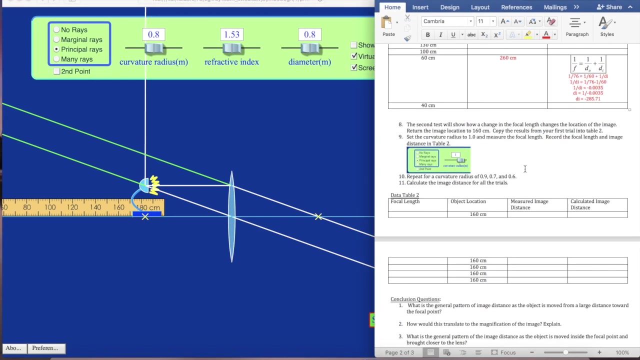 because it's a virtual image. I'm trying to move this screen, but it won't move. Well, that's interesting, Hmm, Okay, anyway. Now it says the second test will show how a change in focal length changes the location of the image. 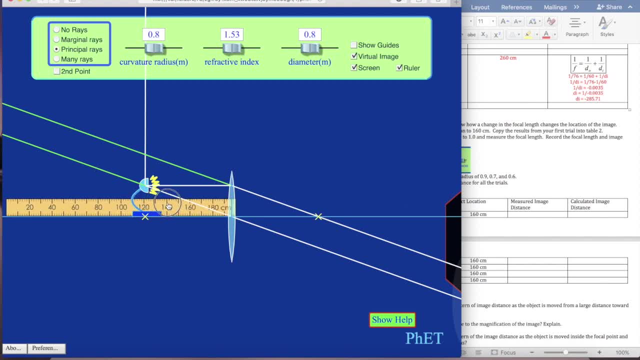 So we're going to return our image location to 160.. Okay, so I'm going to put 160 at the center of the lens and I'm going to put my image where it starts. See all the rays. Okay, Because I want them to start, like, right at the edge of the ruler. 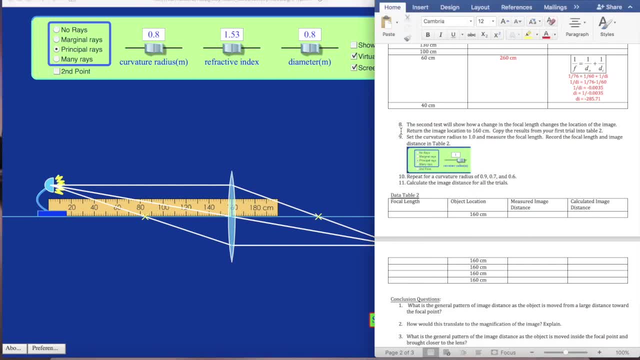 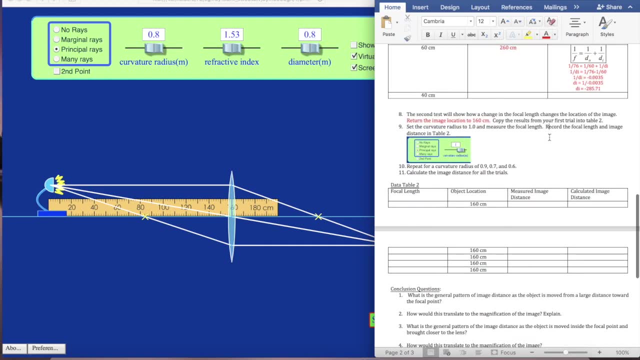 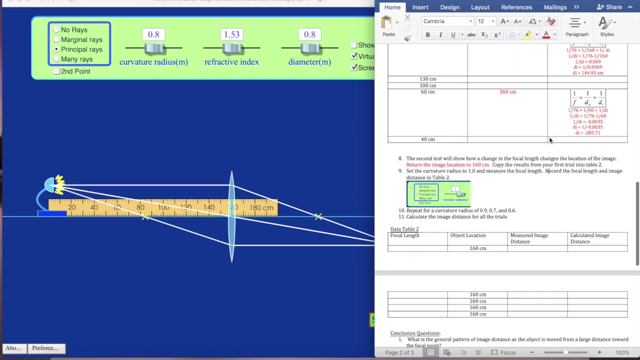 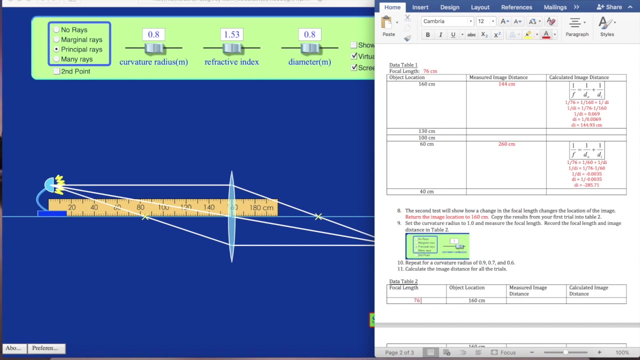 So that's about right. And then it says: copy the results from your first trial into table two. Okay, Okay, so they want, like I'm going to put my image here. This was like if your focal length was 76,. 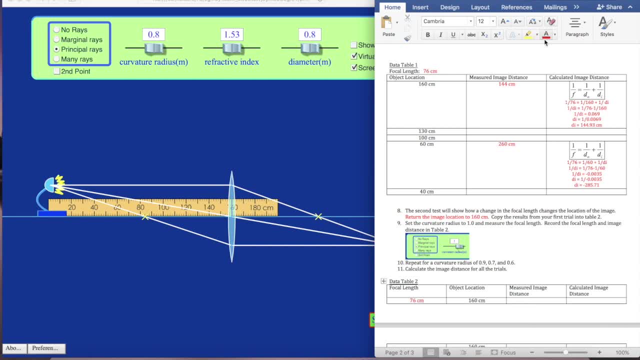 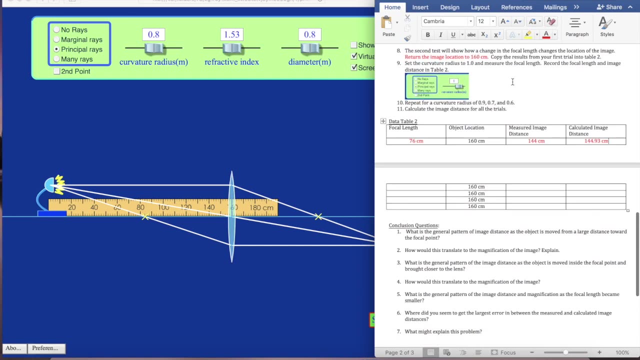 then your measured image distance would be 144, and then your calculated image distance would be 144.93.. Okay, so that's what they wanted me to record. Okay, then it says: set the curvature radius to 1, and measure the distance to 1.. 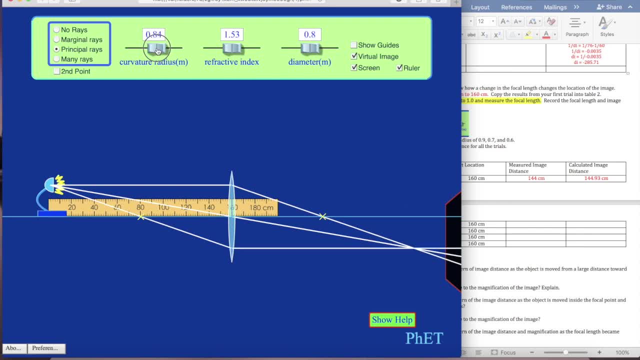 And now I'm going to measure the focal length. Okay, so the curvature radius. I'm going to move this to 1.. And now I'm going to measure my focal length. Okay, so I'm going to take 0 at the center of this X. 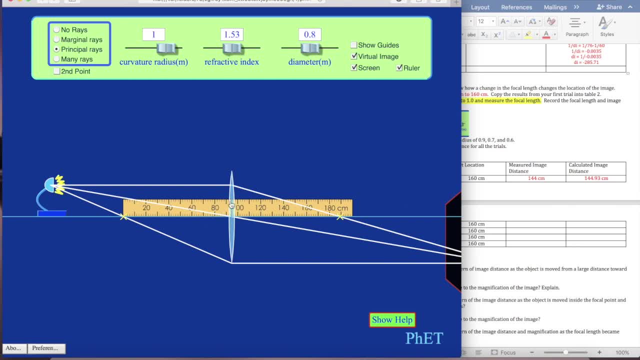 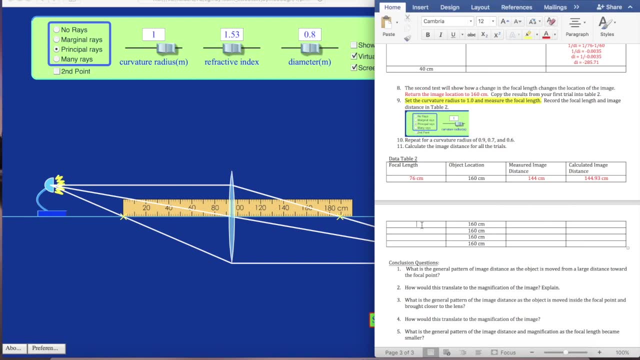 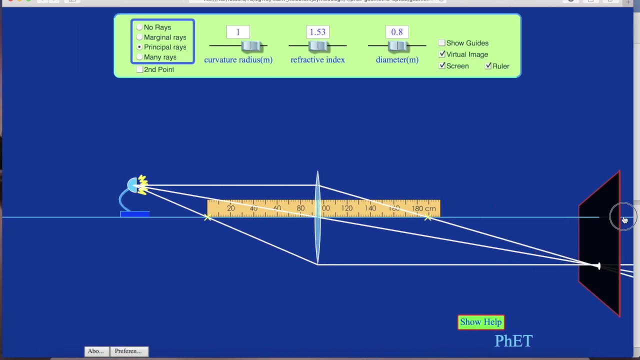 and then I'll measure what we've got here. So we've got like what, 92,, 94,, about 94. 94. Um, And then we're going to measure our image distance again. Okay, so our image distance again is going to be where, um. 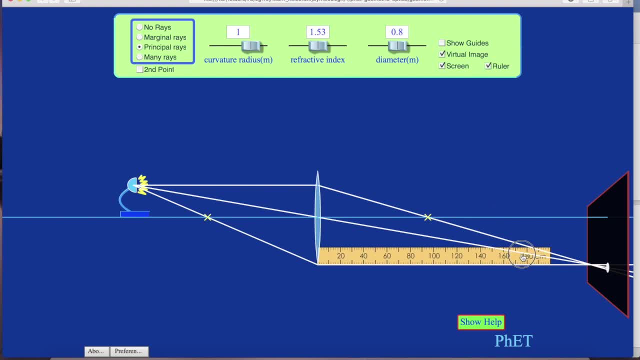 these intersect. So I'm at 200 here, And since it's a little farther than this, I'm going to put my finger here. That way I can, you know, re-measure it. I'm going to move this screen out of the way. 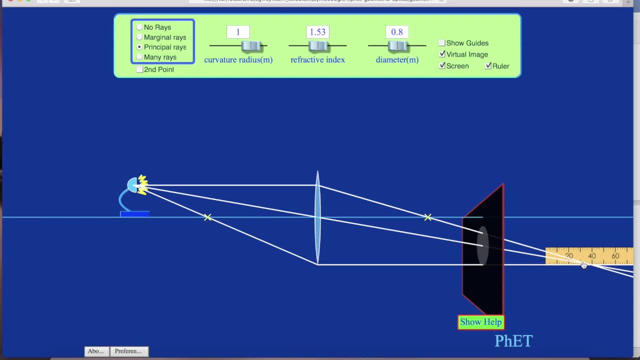 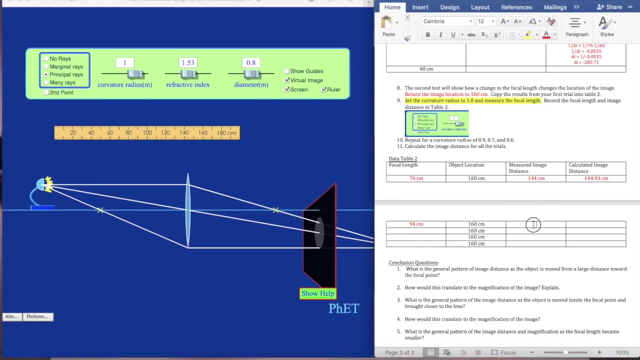 So what we have: 200, 210, 220, 230, 238.. So I'm going to write that here And then, um, we can calculate the distance from here. so we're going to move this to here. 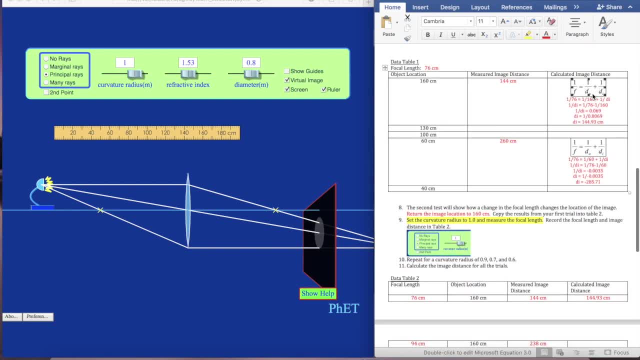 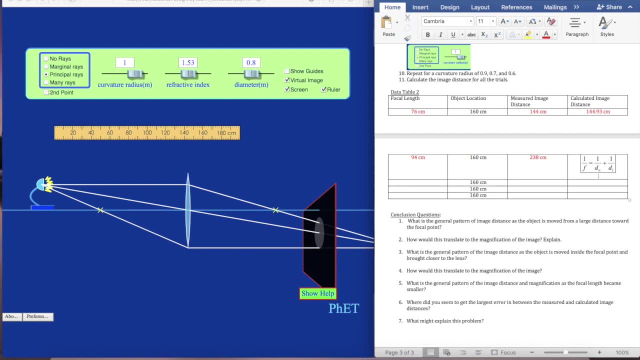 So we're going to move this to here. We're going to move this to here. Okay, the image distance again, and I'm going to calculate it for this one, just because I want to make sure that we did it right. okay, so we have make this red. 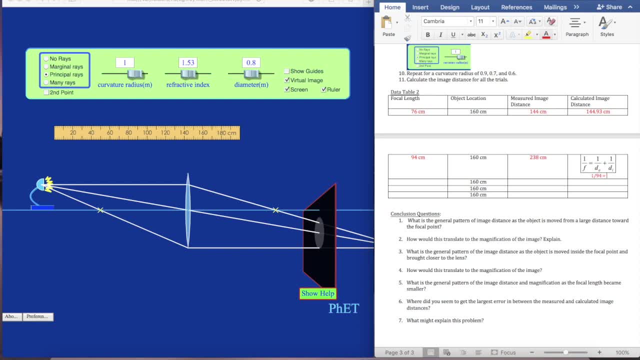 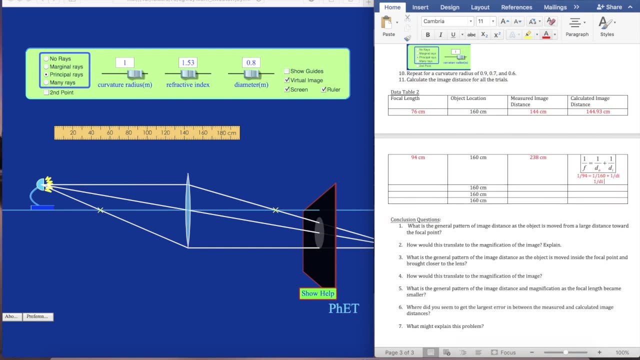 you have 1 over 94 equals 1 over 238, or, sorry, 1 over 260 or 160 plus 1 over di. so then we have 1 over di equal to 1 over 94 minus 1 over 160, so 1 over di is. 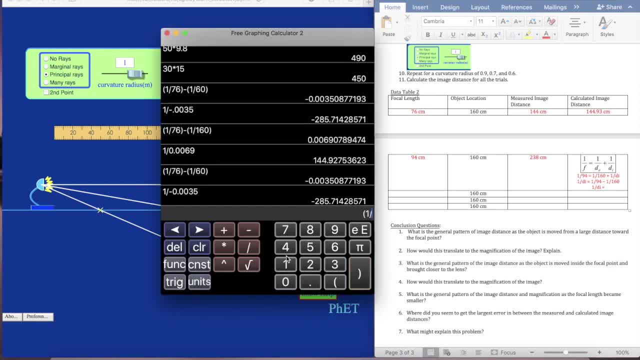 equal to. so I'm going to do 1 over 94. and do you see how I'm putting these in parentheses? this makes sure that I get the right answer, because otherwise sometimes the calculator doesn't know order of operations as well as we do. okay, so I got this. it's a positive number, so at least it's on the right side, it you? 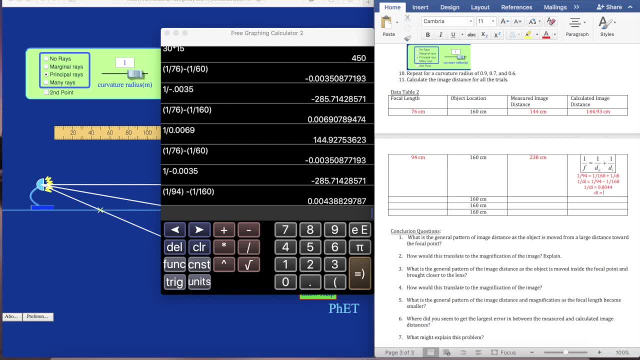 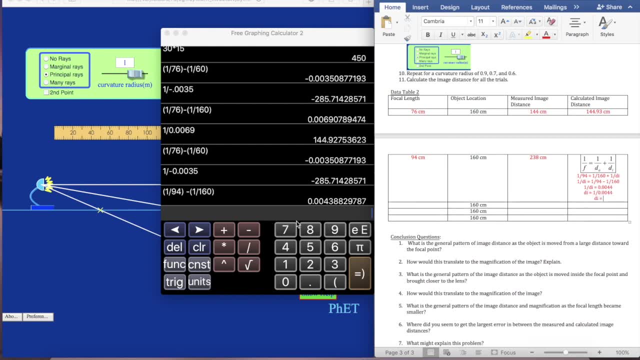 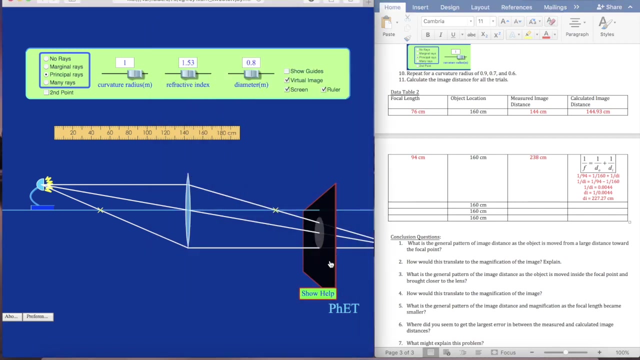 know it makes sense. and then we can do: di equals 1 divided by 0.0044, we get 227. that's not too bad. it's not as close as our other one, but I think what's throwing these off a little is probably my fingers a little fatter. then you know if 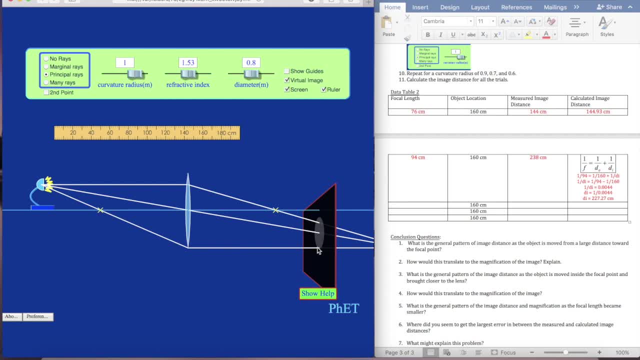 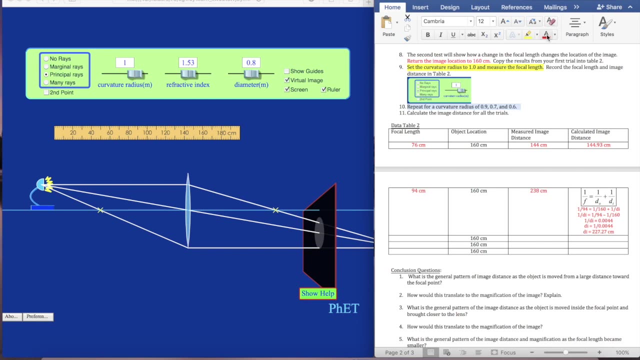 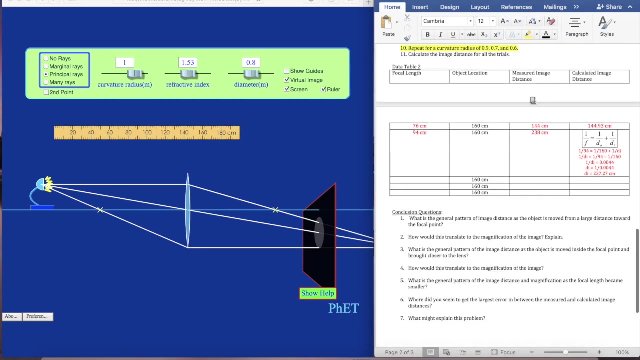 I could do like the mouse point. but if I put the mouse point here then I try and put my ruler there. you know it's, it's gonna move, the mouse point going to get the ruler. so that's why I don't want to asking you guys. situation's all the cleaning up here, videos acting like no. 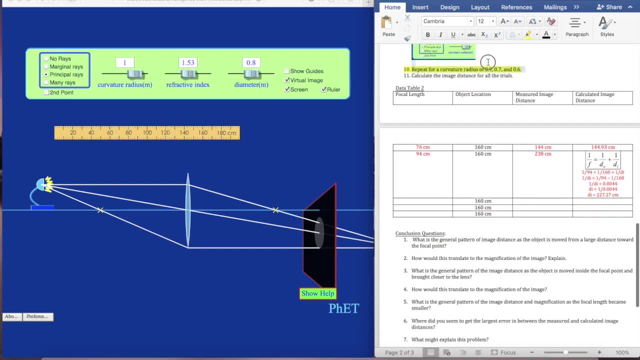 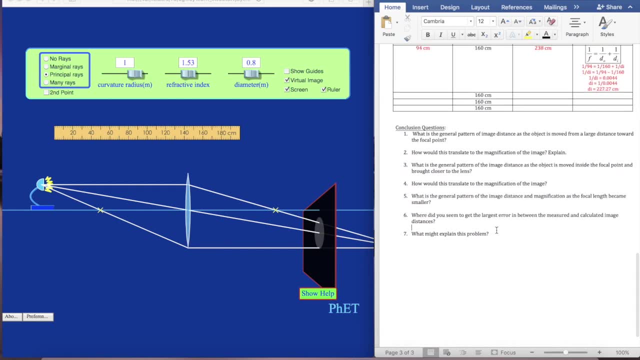 special you coffee right. everyone does get everything it needs to work, exactly right. so this is so I'm going to go ahead and fast forward one for you. and then there's some conclusion questions. okay, here's a hint. when it says explain, you can't just say like yes or no, or you know you have to.